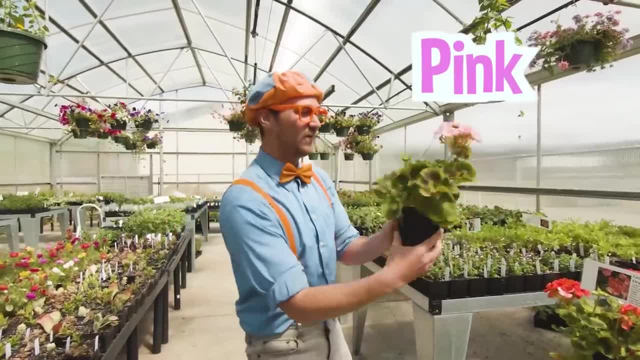 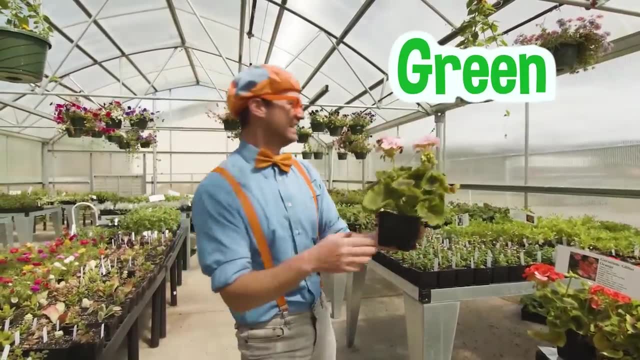 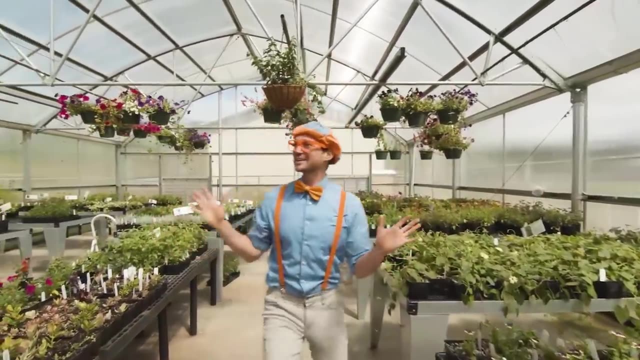 Yeah, It's the color pink. Ooh, And all these leaves. What color are they? Yeah, The color green. Wow, Flowers are so cool. You can put them on your tabletop and they look so pretty. Whoa, What kind of plants are these? 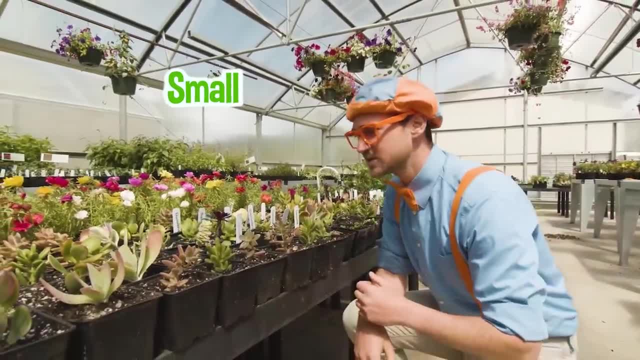 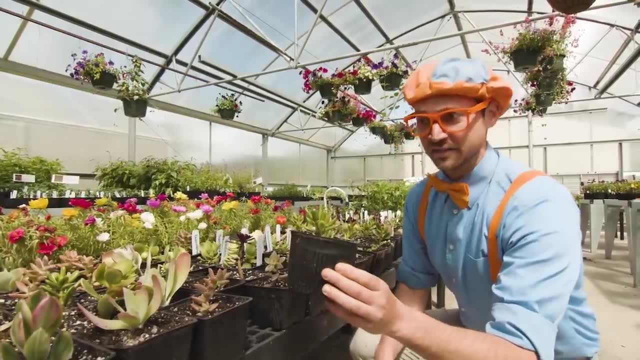 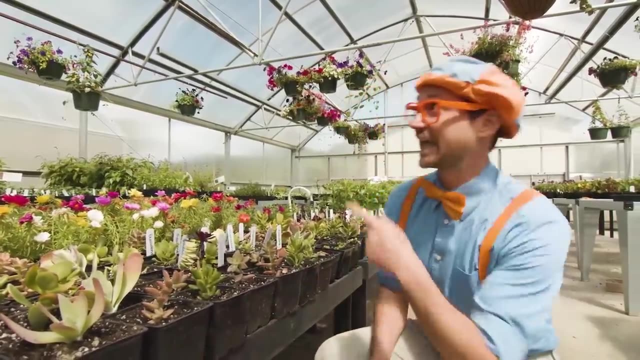 Whoa, They look real small compared to those flowers. Yeah, These are actually called succulents, Huh, Interesting. Hmm, They kind of look like cactuses, Yeah, But they're not pokey or anything. Actually cactus. 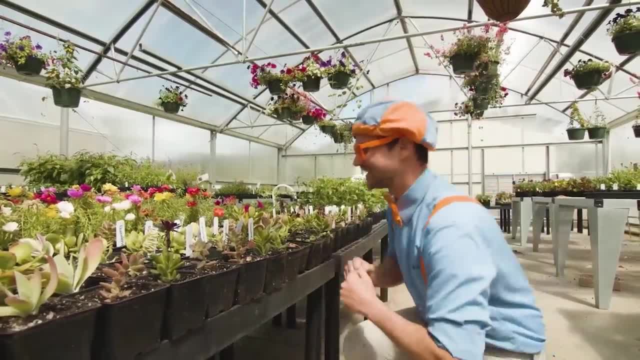 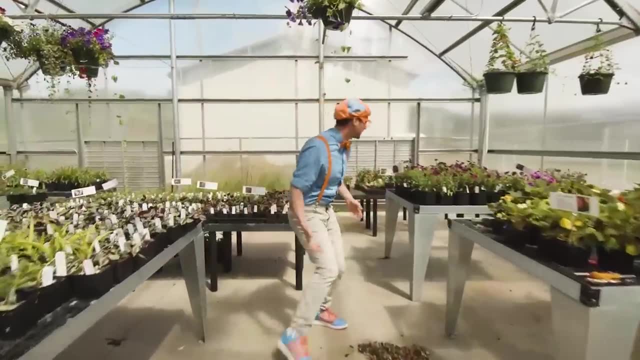 Yeah, That's a type of succulent. Wow, Succulents are so cool. Whoa Ooh, Some more flowers over here. Wow, There's so many flowers. A lot of greenhouses have flowers in them, Or they could be growing fruits. 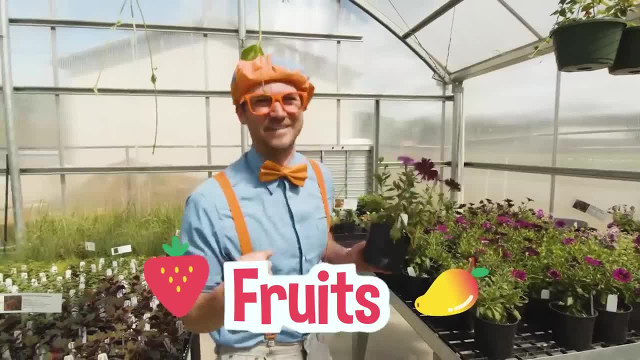 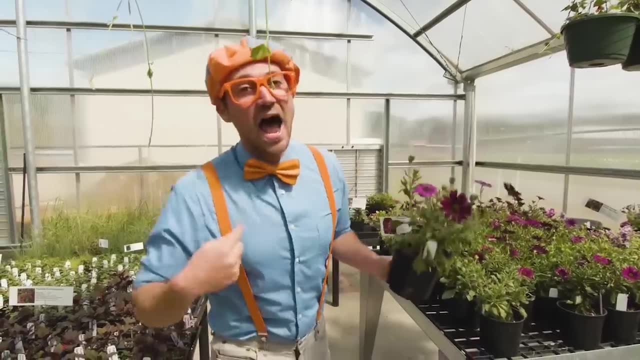 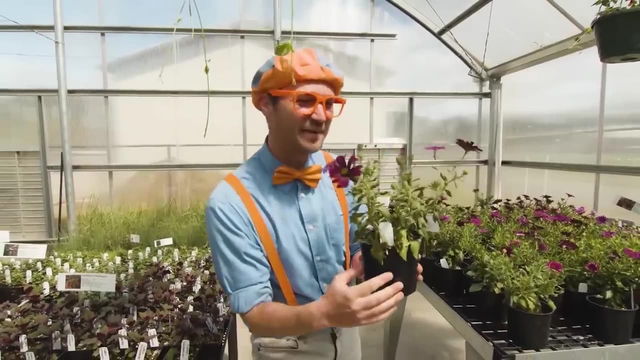 Hmm, I love fruits And I might grow vegetables. Yum, I love vegetables too. I really enjoy eating healthy. Do you eat healthy? Yeah, Good job, Yeah, Good job, Yeah, Good job. But hey, What color is this flower? 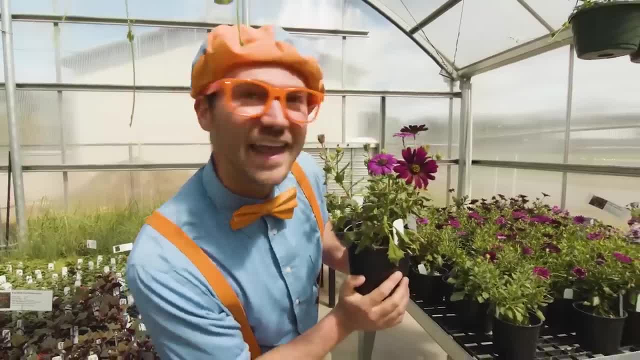 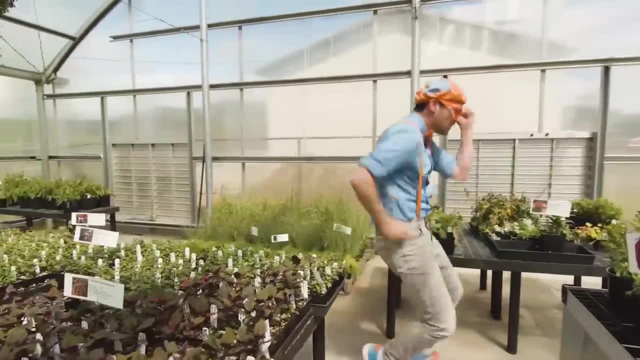 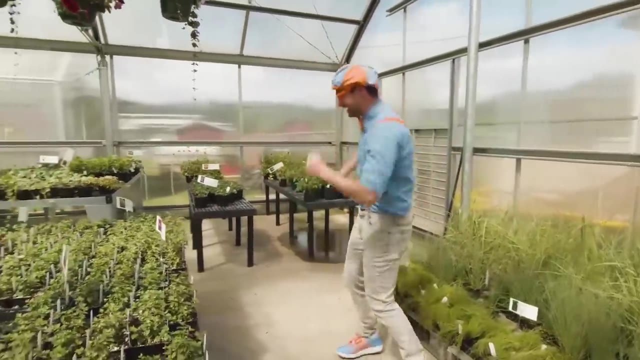 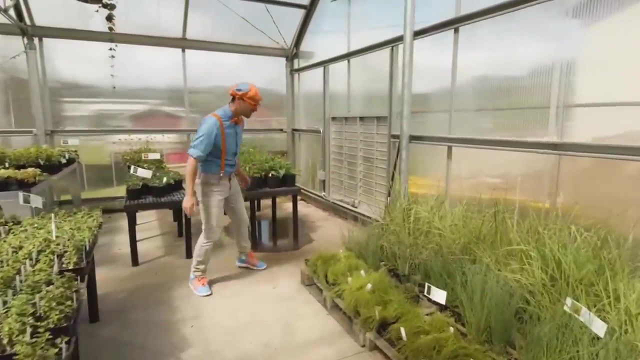 Yeah, It's the color purple. Yeah, It's the color purple. Yeah, It's the color purple. Come on, Come on, Whoa, Check it out. Some more plants. Do you see these kind of plants? Yeah, It's not a flower. 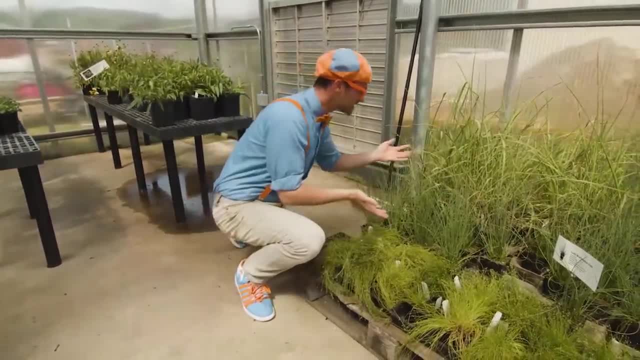 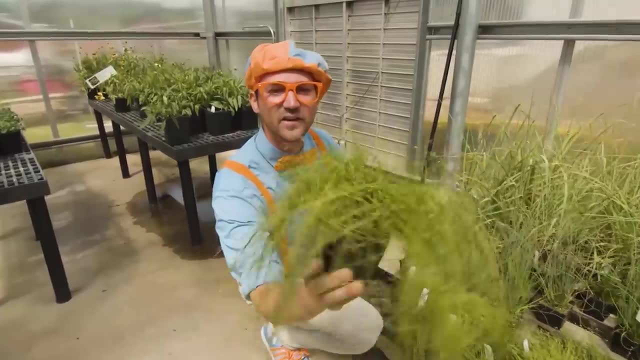 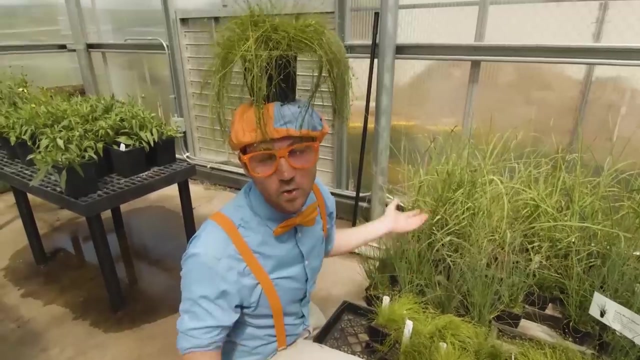 It's not a fruit, It's not a vegetable. These look like a type of grass. Yeah, Three different types of grasses. Look, Whoa. Looks like my hair. Hello, Hey, Do I look silly Or do I look silly? 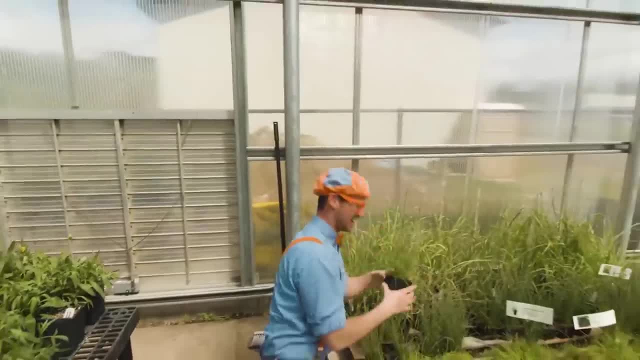 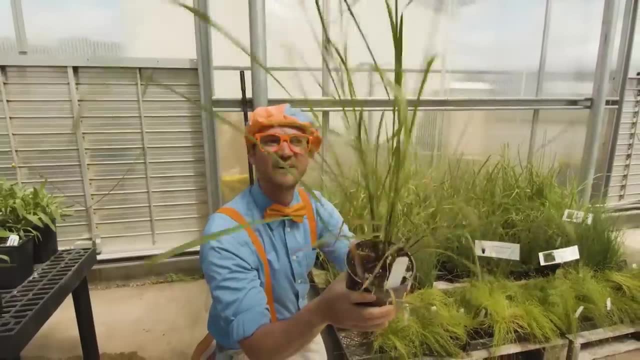 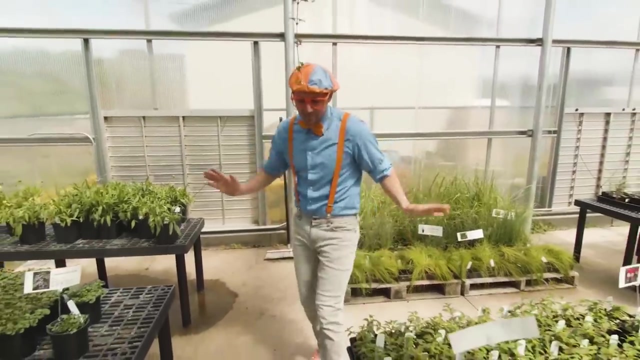 Now that is silly. Here's another type right here. Here's another type right here: Whoa And another type, Whoa. Yeah, Do you have grass at your house? You very well might. It's so fun to play in. 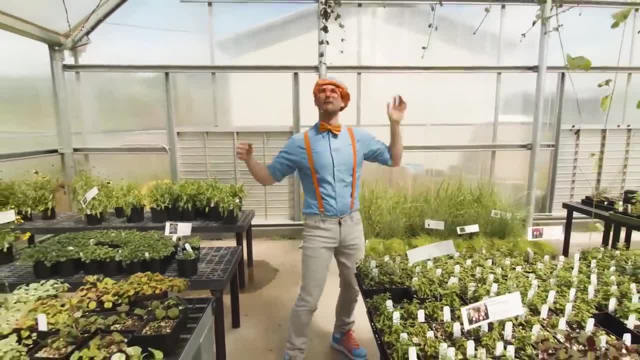 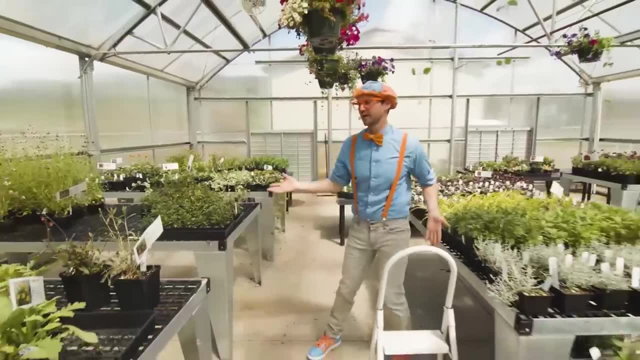 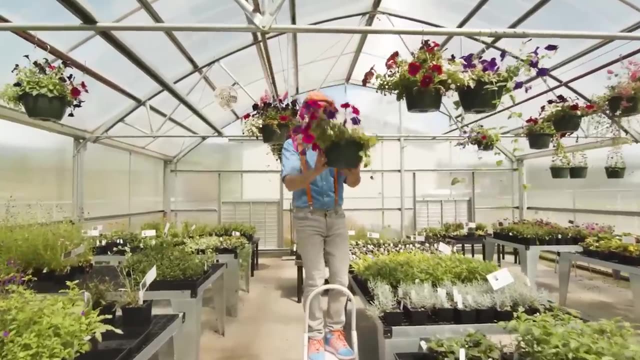 And roll in Whoa, Whoa, Whoa, Wow, Oh, There's so many plants in here. I enjoy greenhouses. Whoa, Look at this. Whoa, Wow, Whoa, A big pot of flowers. 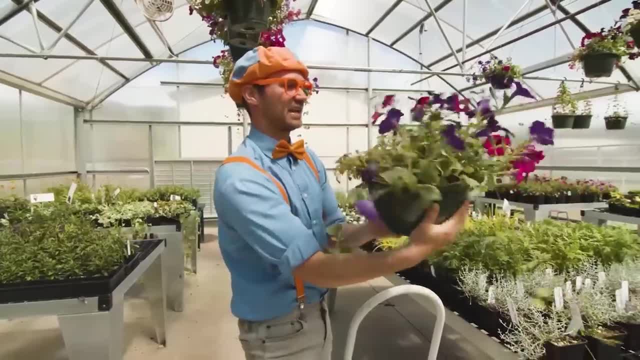 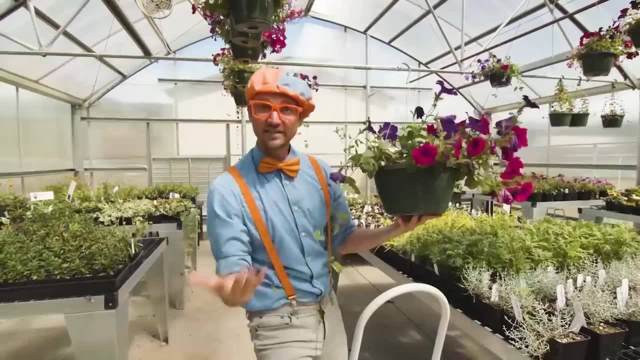 Did you see how it was hanging? Yeah, This looks like a nice, pretty bouquet of flowers. Yeah, A bouquet is where it's a big group of flowers, But typically you cut them off and then you can make a very colorful bouquet. Wow. 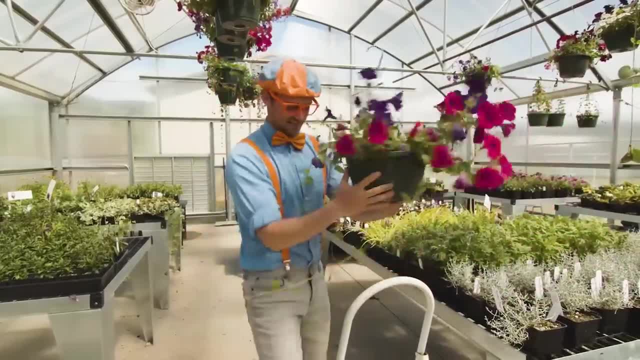 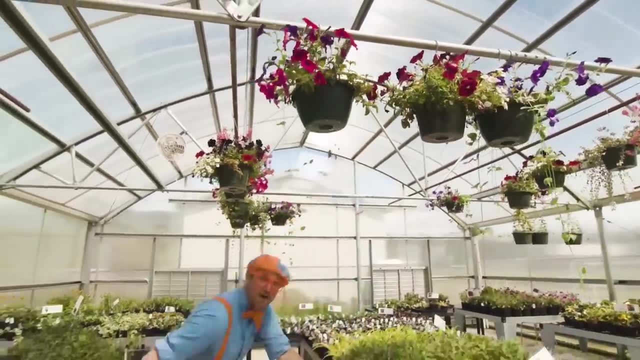 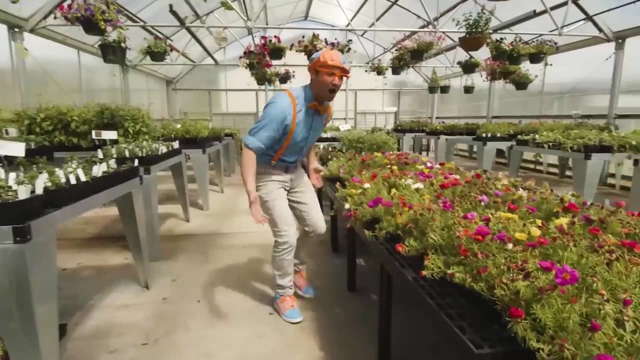 So pretty. But this is also pretty and it's in a hanging pot. Wow, We have to make sure we put things back where we found them. Woohoo, Whoa, Check these out. Wow, So many colors. What colors do you see right here? 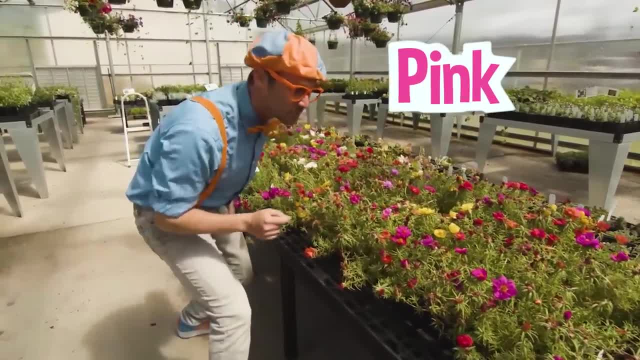 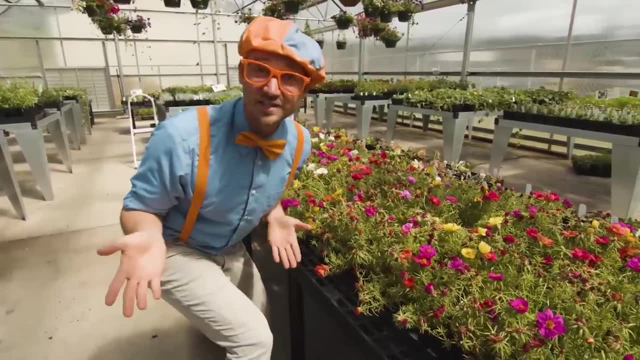 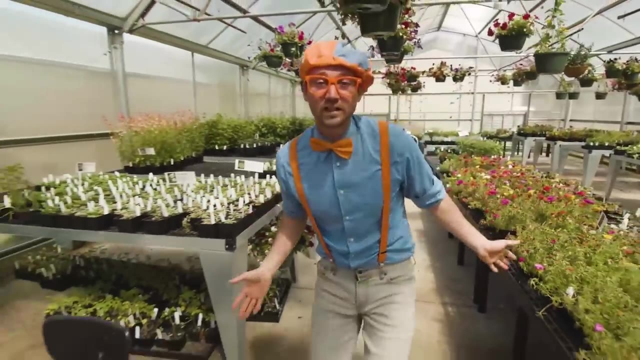 Looks like that one is pink. That one right there is red. Ooh, Look at that one. It's the same color as the sun. Yeah, Yellow, Whoa. Alright, I have a really fun thing for us to do together. 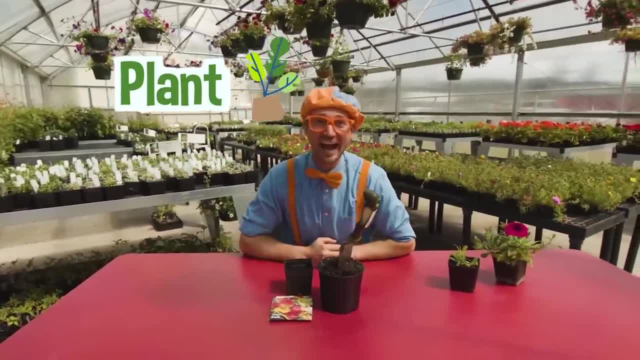 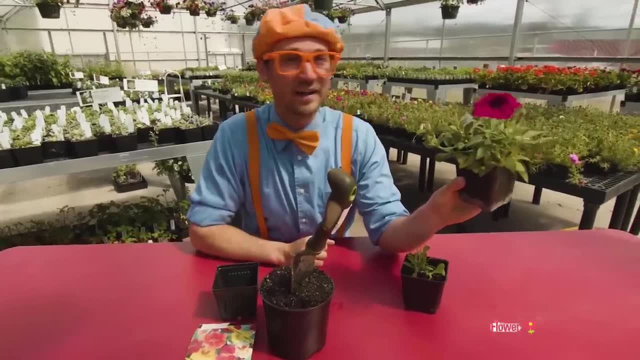 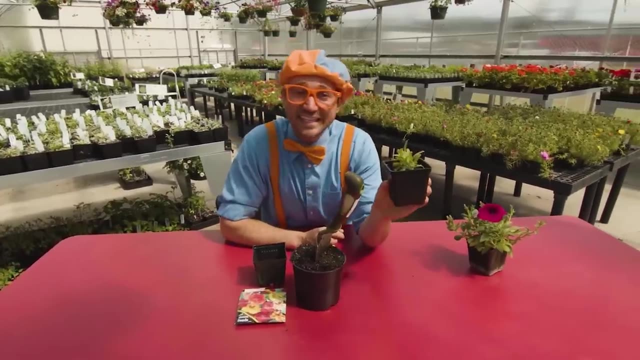 Have you ever planted a plant? Yeah, It's so much fun. Do you see this? Yeah, You know what this is. It's a flower. It's an adult flower. It's really old. And look at this one. This looks like a teenager. 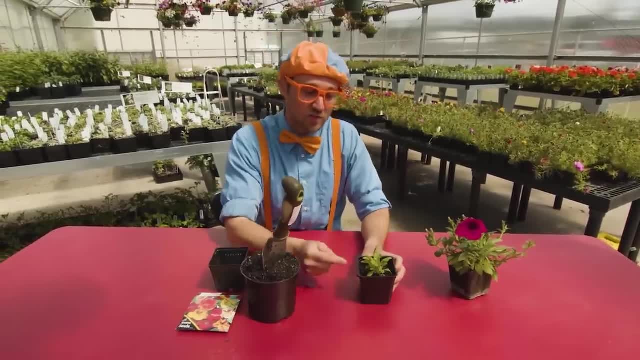 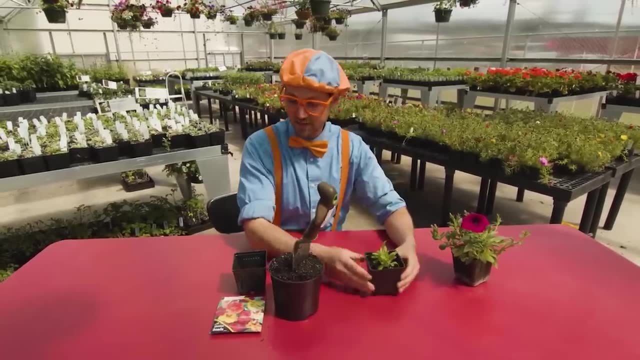 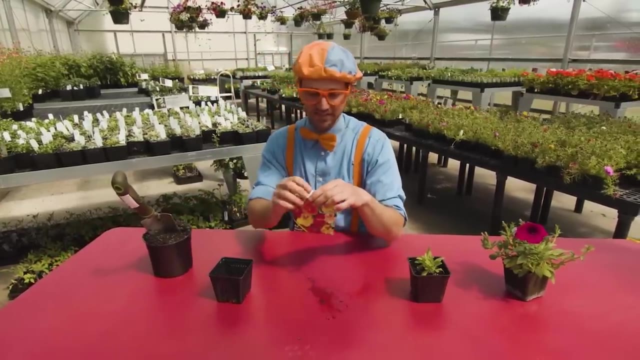 Or a baby. It hasn't even created the flower yet, But soon enough it will turn into this. But in order for it to become this size, Yeah, It starts out as a seed. Yeah, Every single plant Like flowers, I should say. 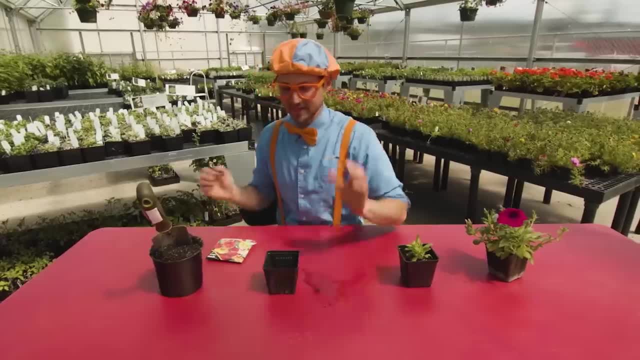 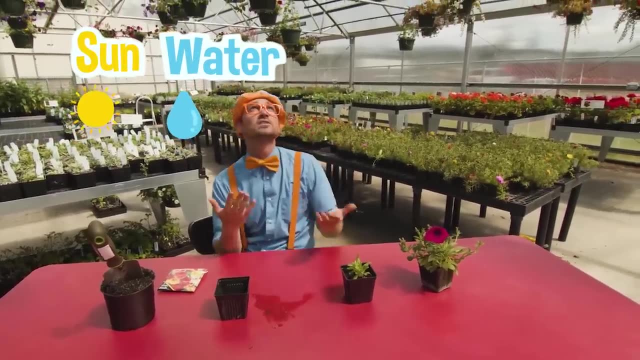 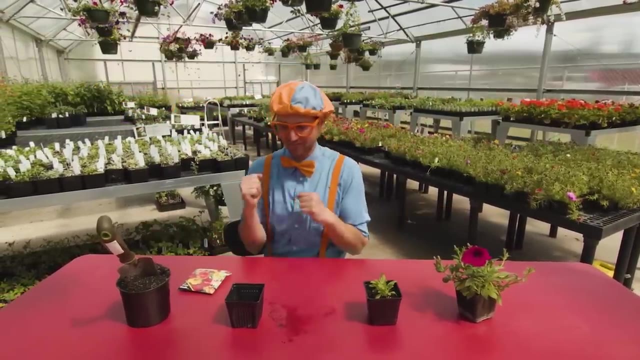 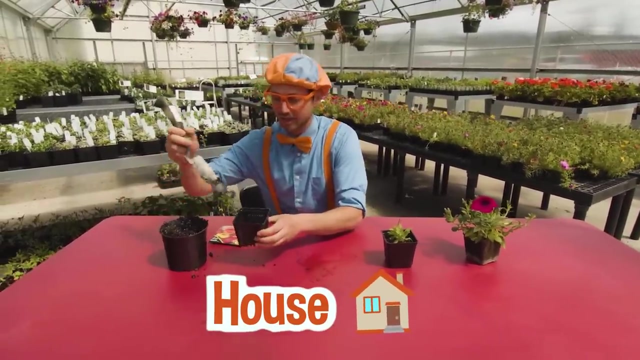 start out as seeds, Alright, But the things that every plant needs are sun, water, soil- which is like a house, and nutrition, Which is like food. Alright, So let's create this plant's house or home, Where we're gonna put the seed. 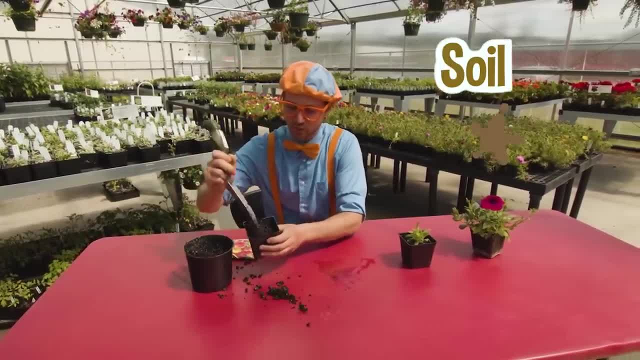 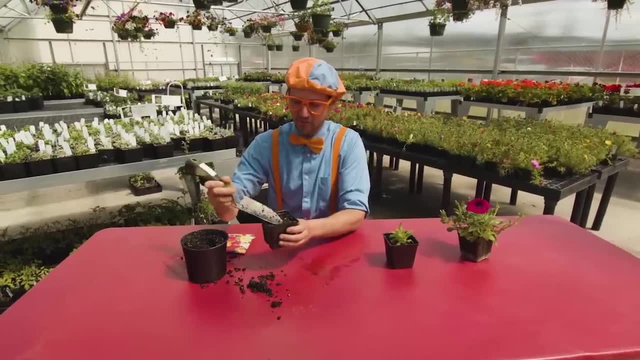 Oh, there we go. Yeah, Let's scoop up this soil. Oh, I'm making a mess, That's okay, I'll clean it up after. There we go. Alright, This soil has a lot of nutrition already in it. 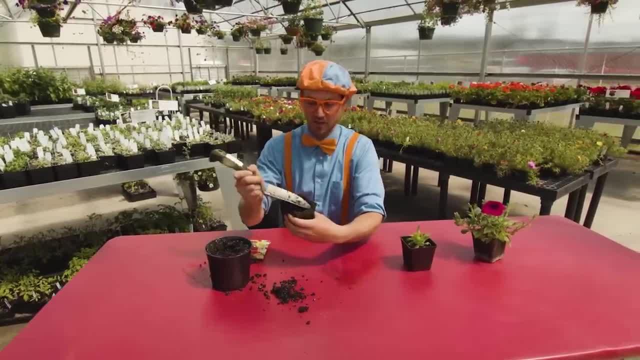 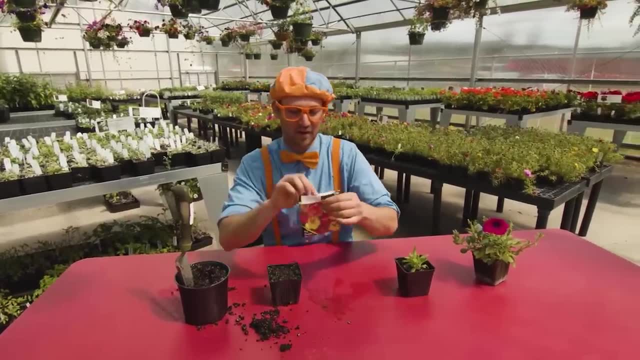 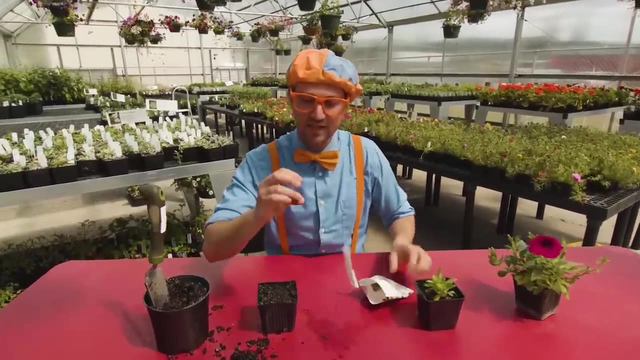 Yeah, There we go, And sometimes the water that you put in this to water, it has some nutrition in it as well. Alright, So check this out. This right here is a flower seed. Wow, Do you see how small it is? 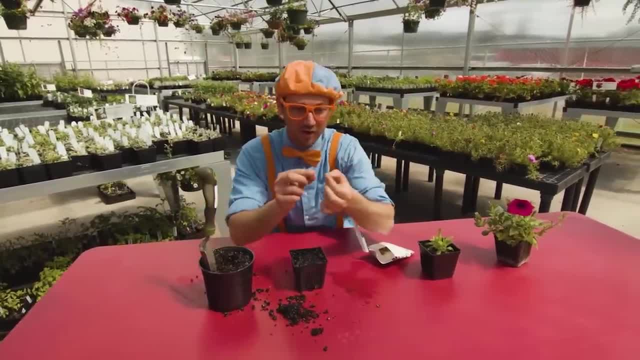 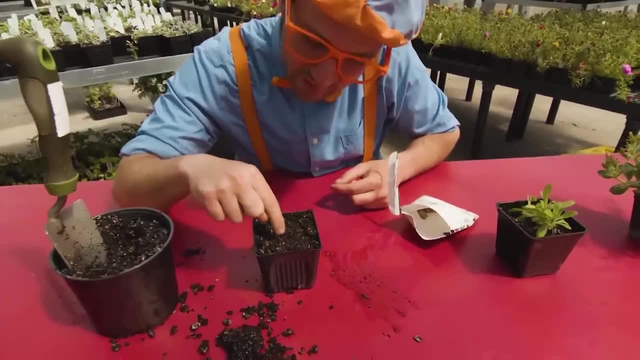 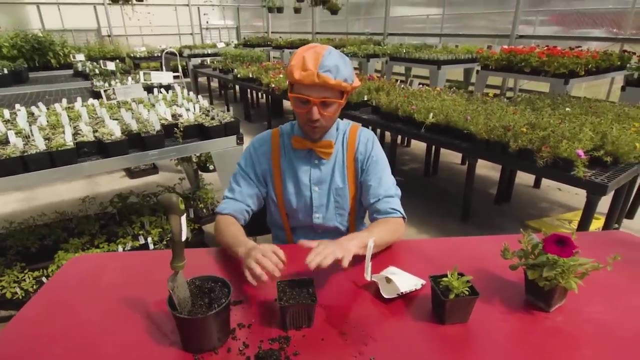 Yeah, So cool. So when you put this right in here and you push it down There, we go: Okay, Let's cover it up just a little bit, The soil is nice and moist, And then after a while it's gonna sprout up. 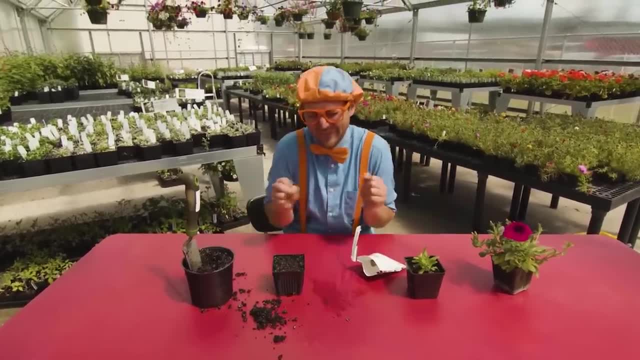 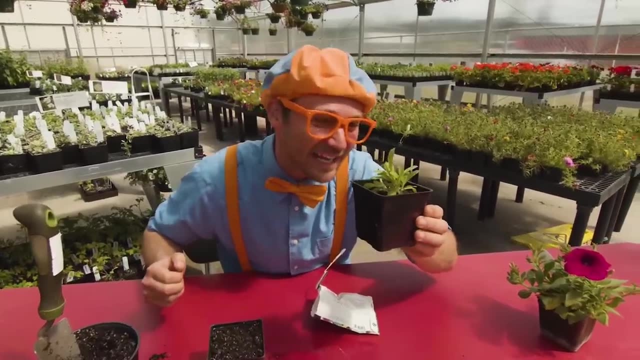 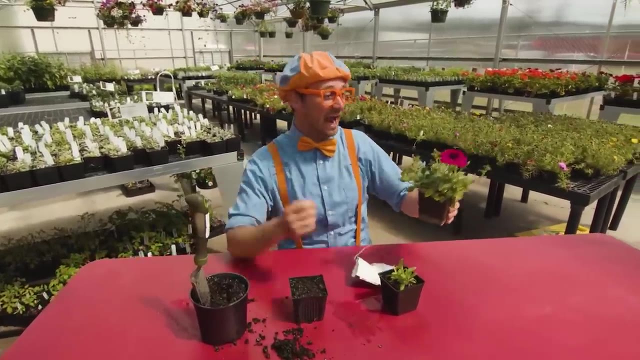 And it's gonna be so small and cute, Oh, And then it'll grow up to be this: Wow, So green and pretty, But when it becomes an adult, it is going to flower. Yeah, Good job, Alright. So what are the four things? 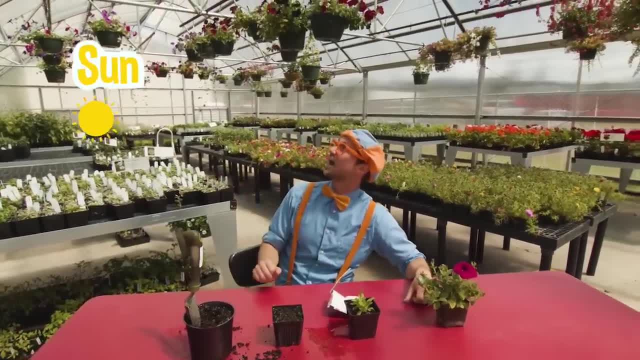 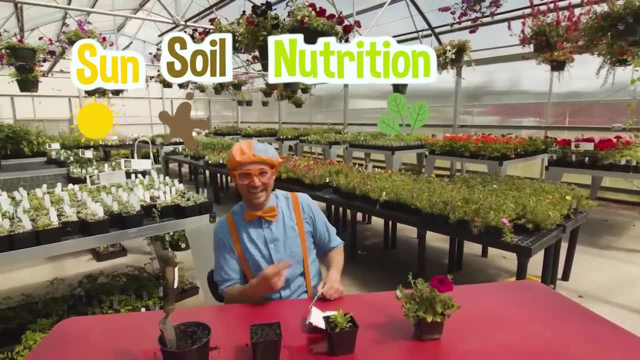 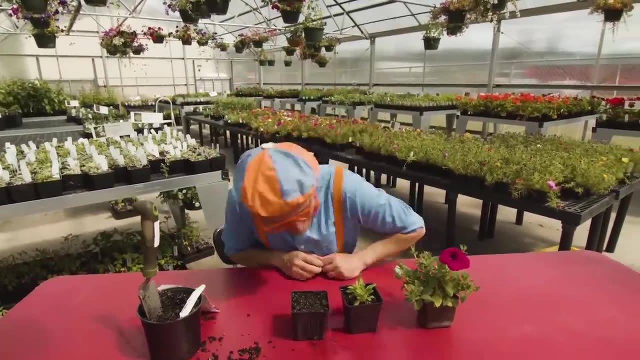 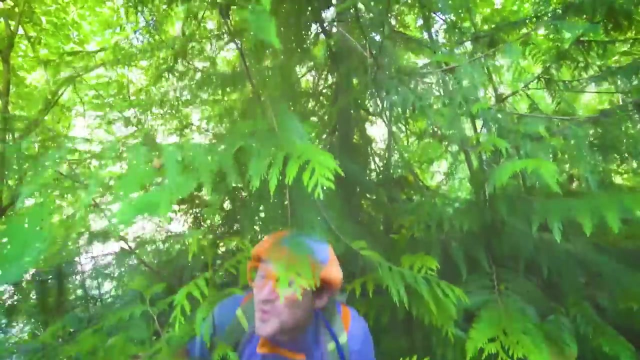 that every plant needs to grow. Yeah, It needs some sun, It needs some soil, It needs some nutrition And it needs some water. Wow, This was awesome Walking through the forest. Look at all the trees. They give us lots of air. 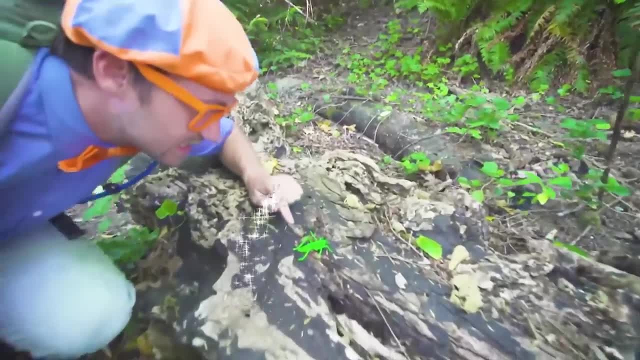 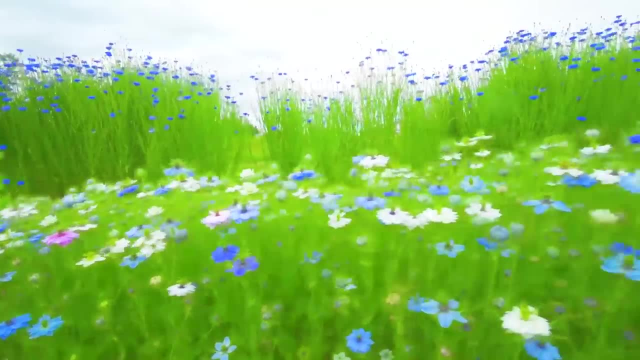 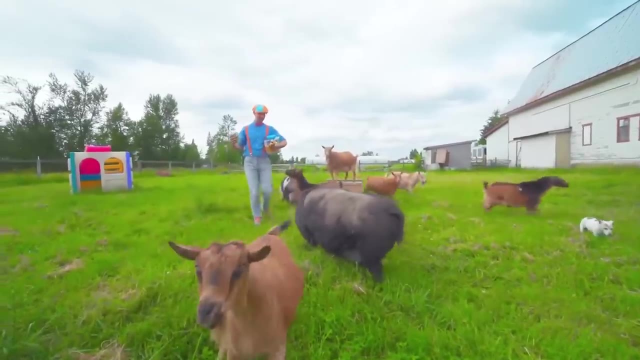 What we need to breathe. Look at all the critters Roaming on the ground. They help carry the seeds To grow plants all around Flowers are a blooming, Making lots of food For all the bugs and creatures, Even me and you. We're singing the Earth song. 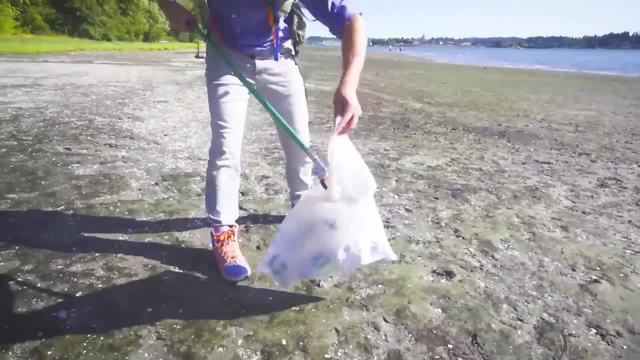 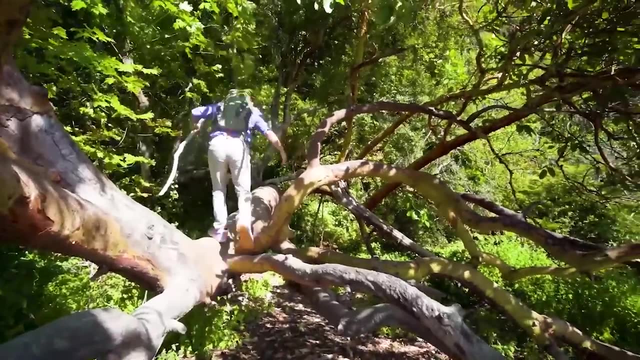 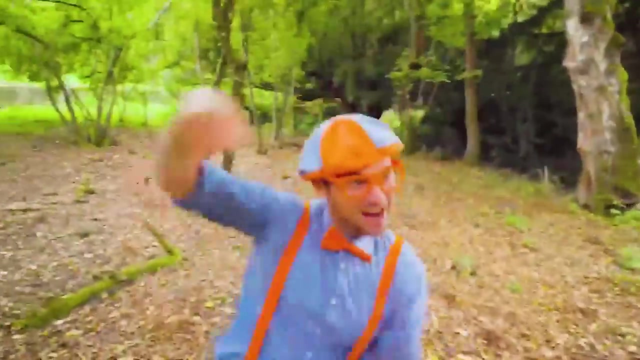 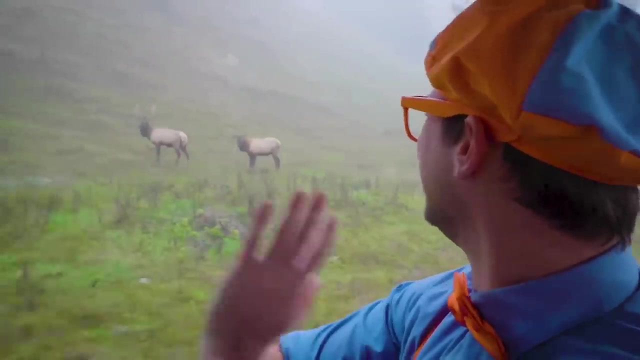 We're helping the planet. Together together, Together together, We can make a change. We're singing the Earth song. We're singing the Earth song. Come learn all about it. Come learn all about it. Together together, Together together. It's time we start. It's time we start. 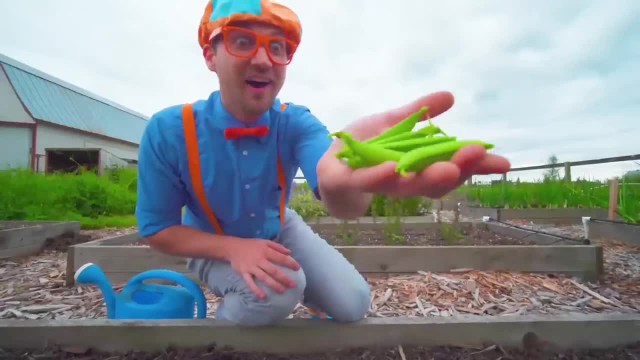 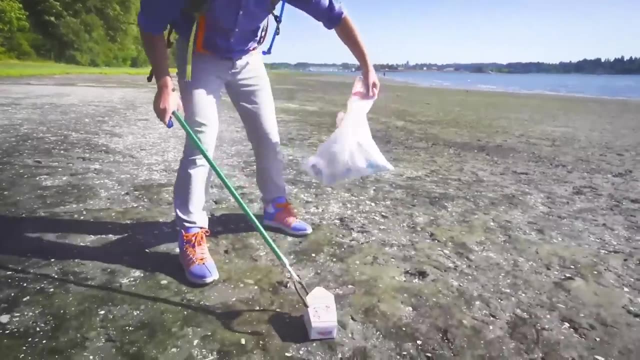 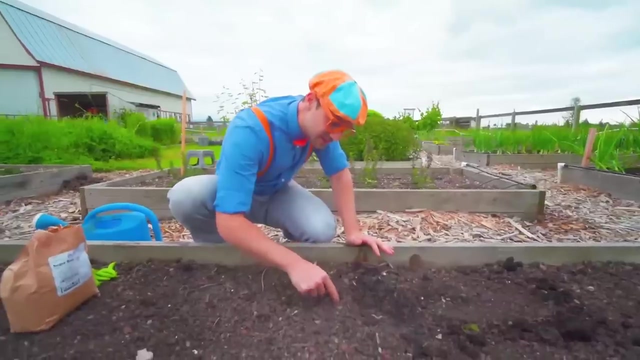 Let's do our part. We can all help Wherever we are. Use a little less water. It goes really far. Make sure to recycle Paper, glass and plastic. Taking care of the Earth Will make you feel fantastic. You can plant a tree Or pick up some trash. 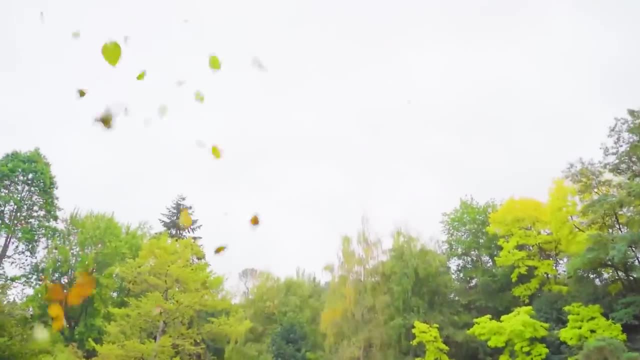 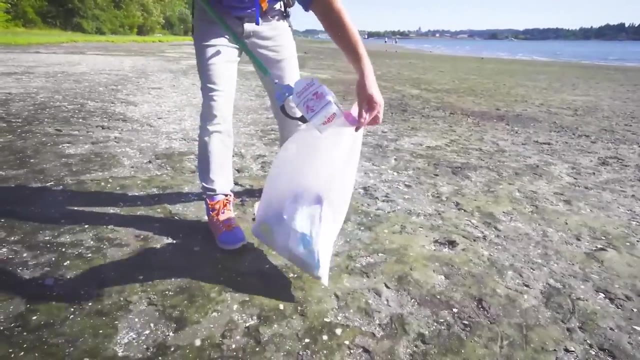 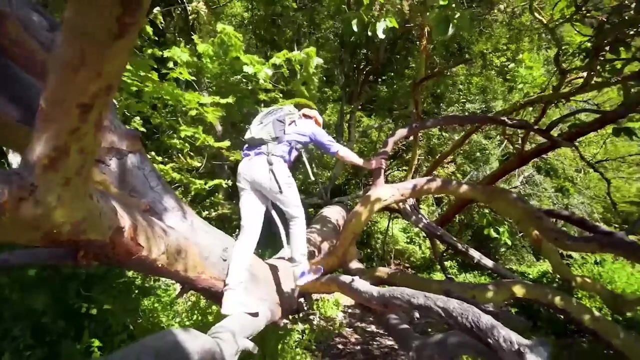 Ask a friend for help, Then it'll be a blast. We're singing the Earth song. We're singing the Earth song. We're helping the planet. We're singing the Earth song. Together together, Together together, We can make a change. We're singing the Earth song. 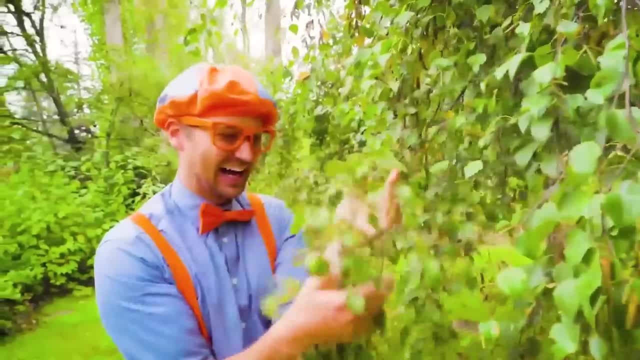 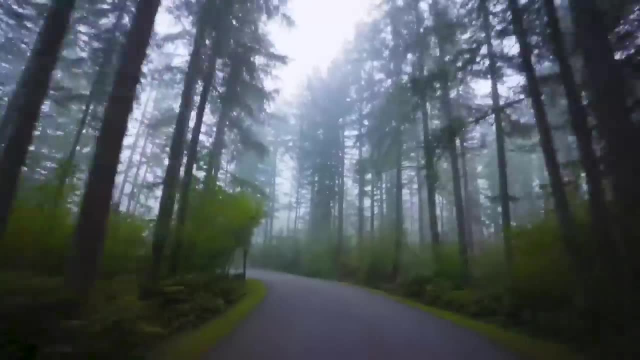 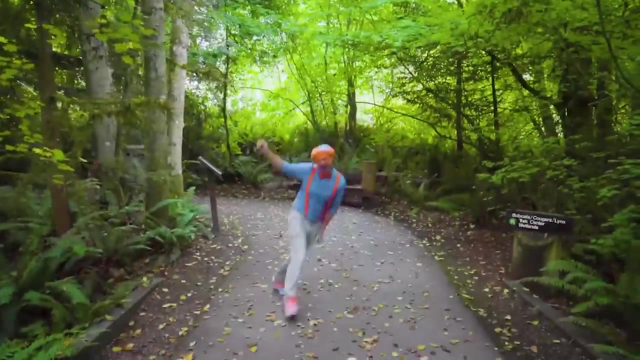 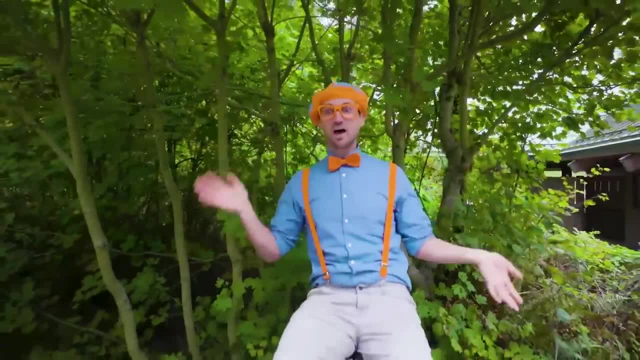 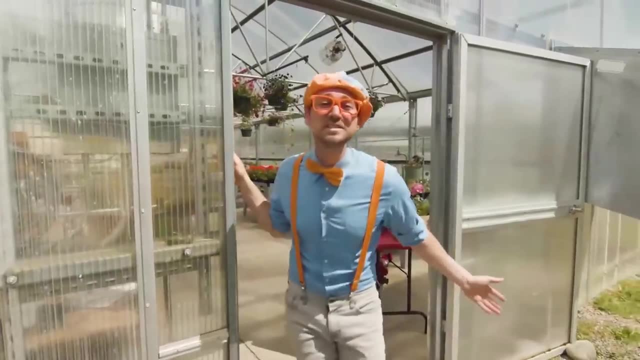 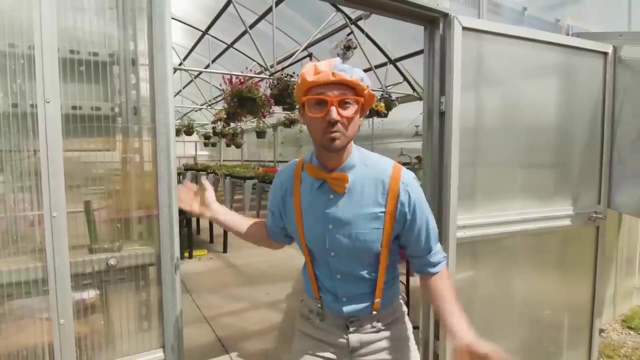 Let's do our part. Let's do our part. That was so much fun learning about plants with you. Well, this is the end of this video, But if you want to watch more of my videos, all you have to do is search for my name. 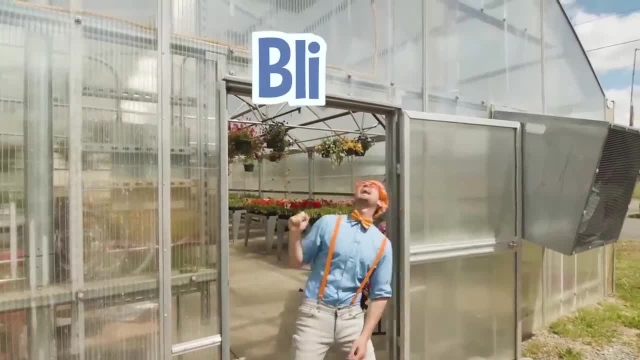 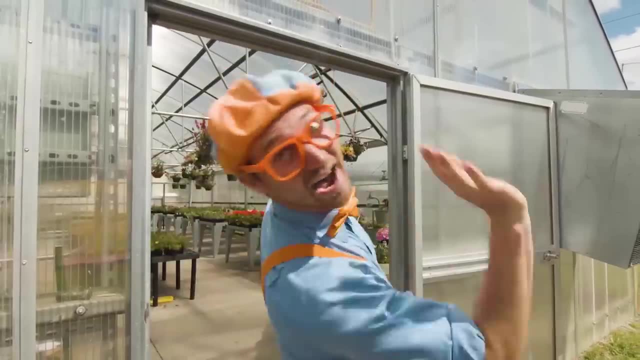 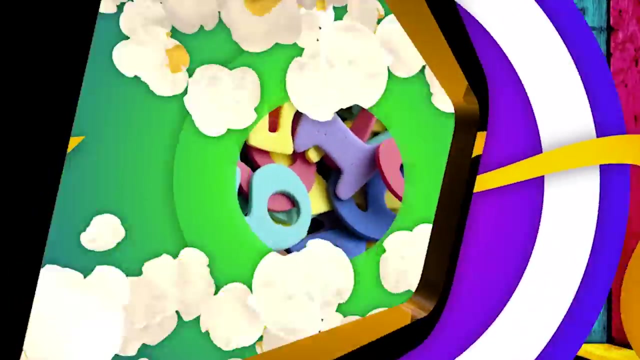 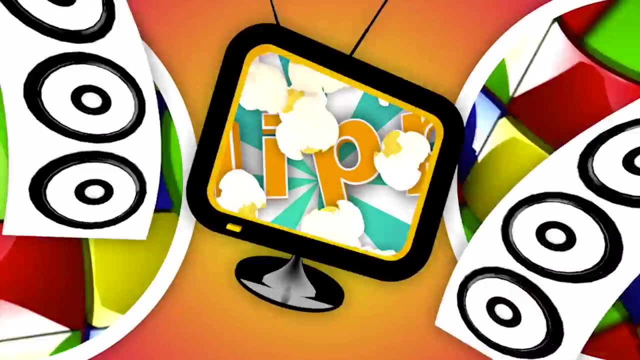 Will you spell my name with me: B-L-I-P-P-I. Blippi, Good job. All right, see you again. Bye-bye, Blippi. come on everyone, let's make learning fun. Blippi, Blippi, so much to learn about, it'll make you want to shout. Blippi.